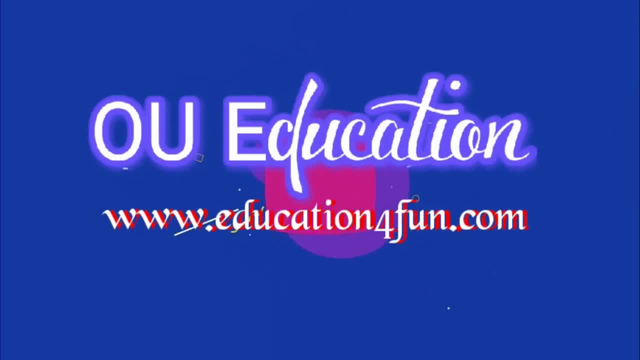 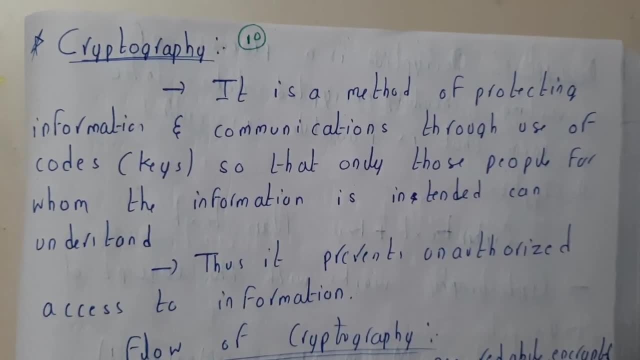 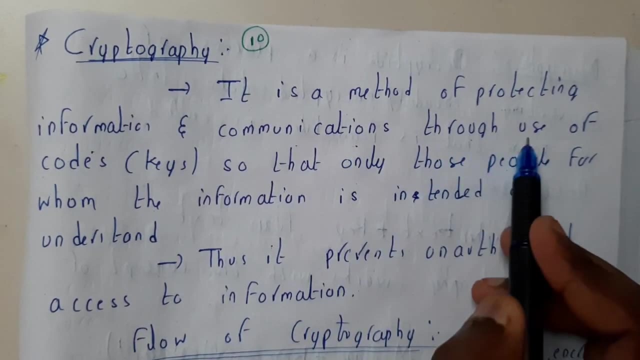 Hello guys, we are back with our next tutorial. In this tutorial, let us go through cryptography. So basically, cryptography it is a method of protecting information and communication through use of codes. Those are nothing but keys, so that only those people for whom the 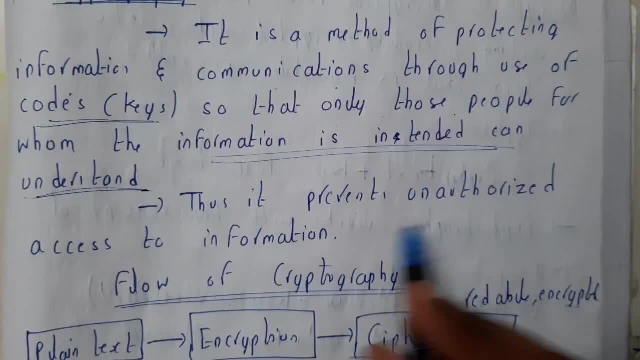 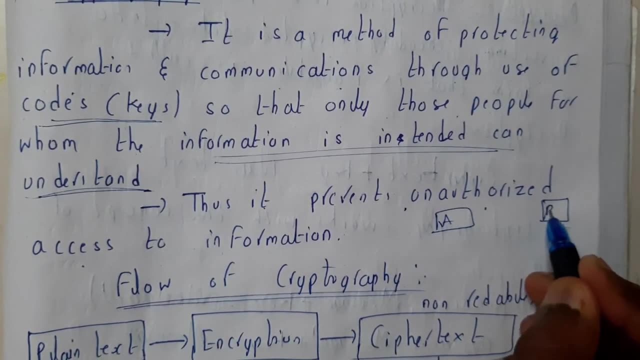 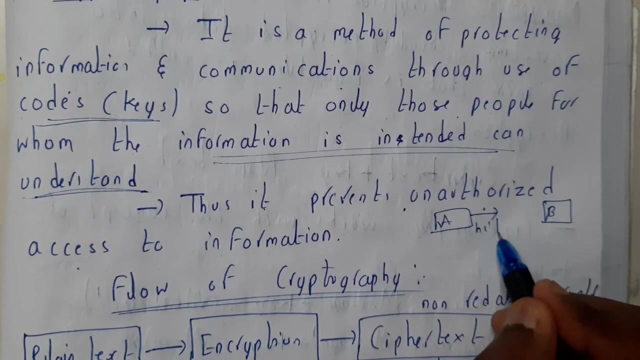 information is intended to send can understand. Thus it prevents the unauthorized access to information. So let us assume I am A and my friend is B. I am sending a message hi to him. Fine, Okay, So if I send a message hi, if there is a hacker or anyone trying to interact. 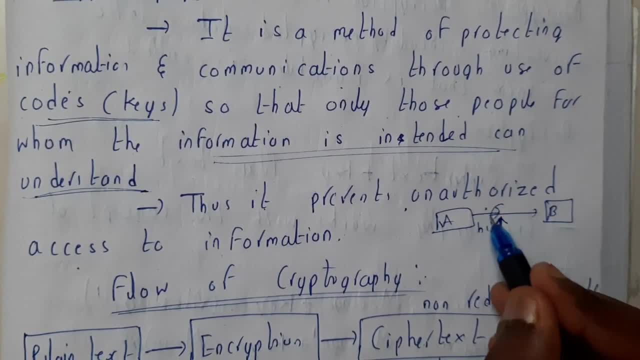 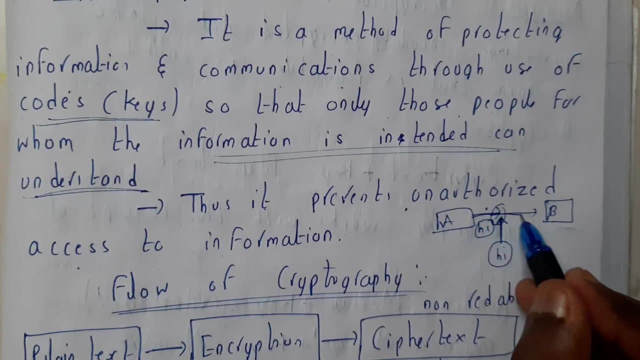 into the medium and if he tries to break the rules and if he can get the message, he will be getting clearly: hi, right, So I am sending it normally, right? So if I encrypt here, so this hi converted into xyz, Whenever a hacker tries he will be getting xyz. He cannot understand it, right? He cannot. 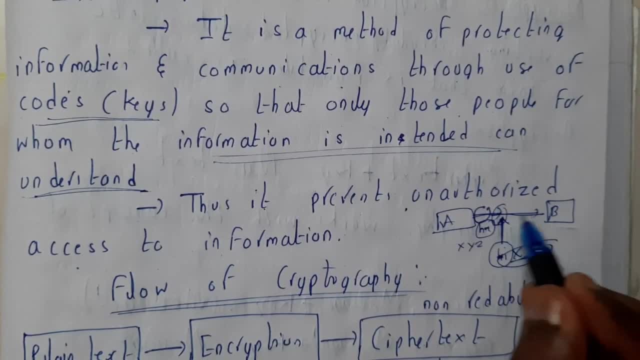 encode it. So that is the reason why he cannot understand the language. Once my friend receives it- before receiving only the decryption will be done and the original hi message will be sent to him. So my message has been sent successfully to my friend without any problem. 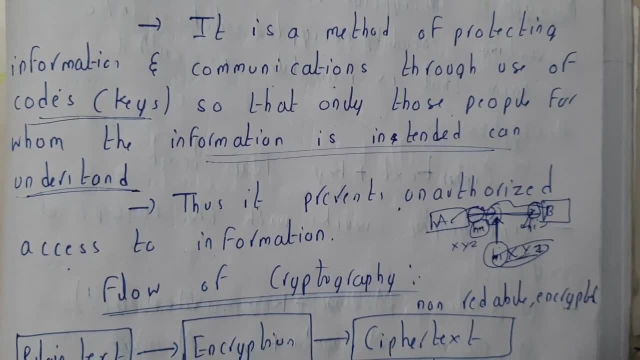 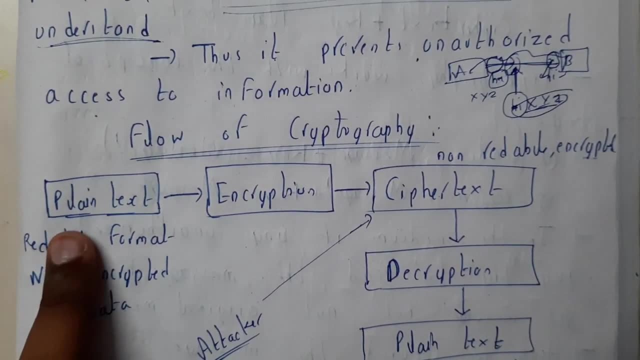 So this concept is nothing but cryptography. I hope everyone got a small idea I have just told you in a small story. Okay, Basically, the flow of cryptography will be in this way: Plain text that is nothing but readable format which a human can read, which is non encoded. 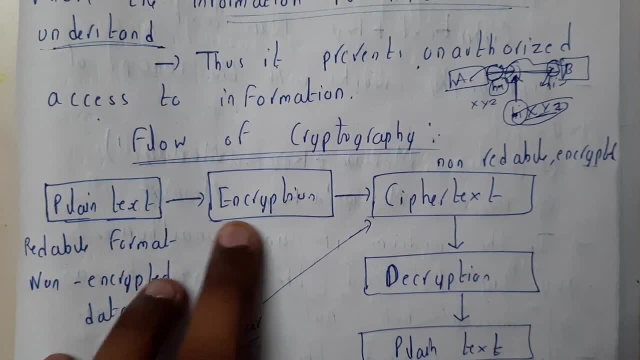 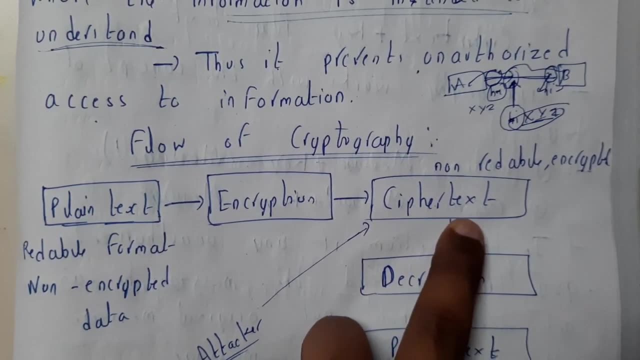 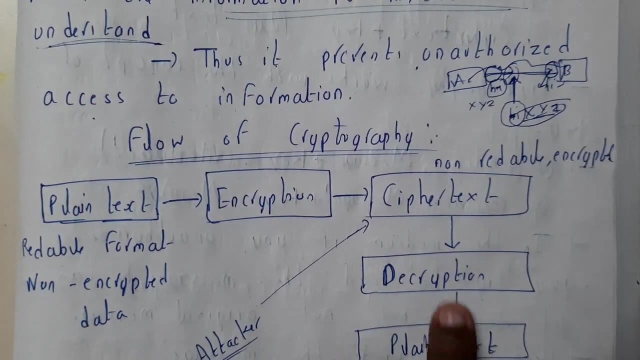 data This: when you transfer it to encryptor, it's going to encrypt the data and that data will be called as ciphertext. Please remember the word, guys, because even I will be forgetting it: It is ciphertext. So ciphertext is a non readable encrypted data. Fine, And this data? 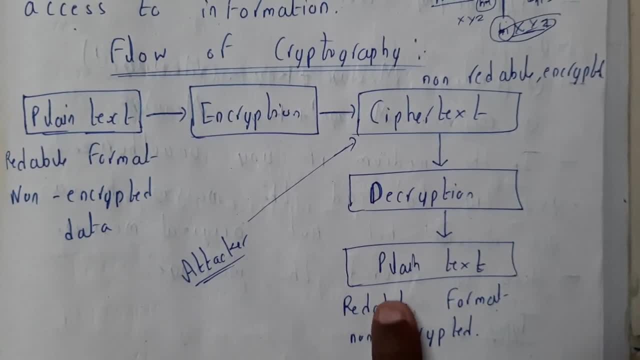 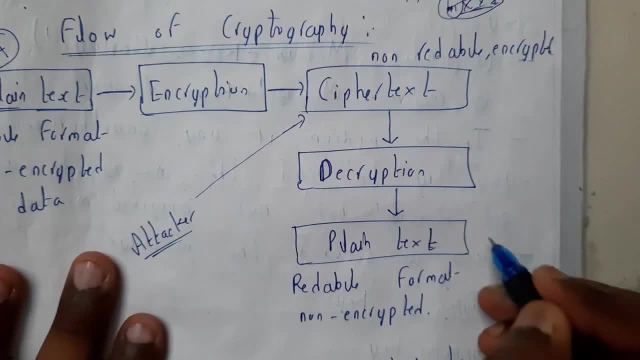 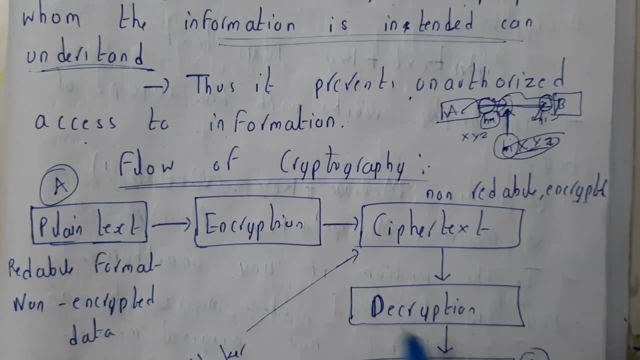 This is the ciphertext, This is this. This is the risk that will be sent from. send endure a to receiver: be fine. So at the end also, it is in the readable and non encrypted format. So where will the hacker be attacking? He will obviously be attacking in the medium. 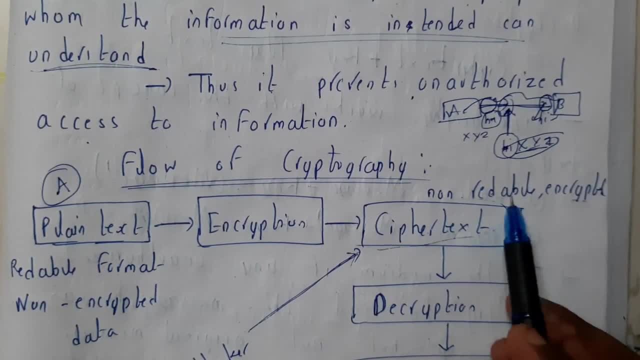 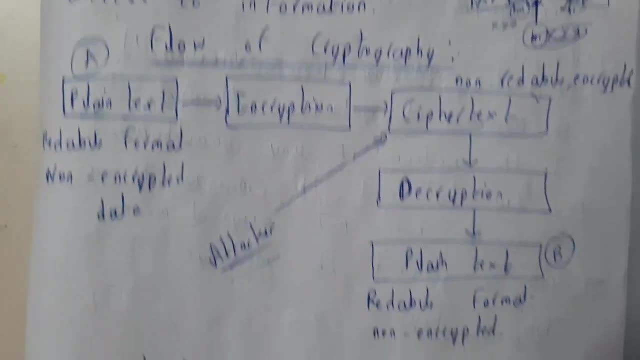 that is nothing, but he'd be getting the ciphertext. The ciphertext is non readable, so the attacker or hacker cannot understand the language. So now let us go to what is encryption and what is decryption. So encryption- encryption- is a process which transforms the original. 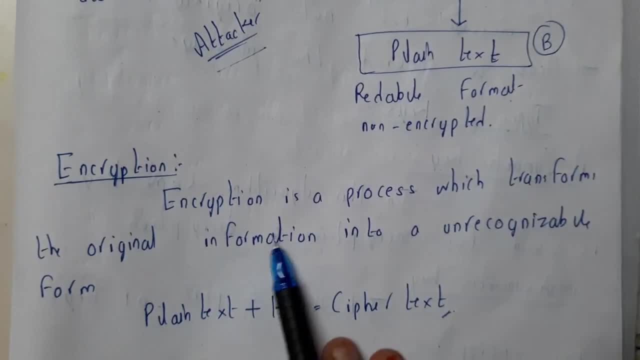 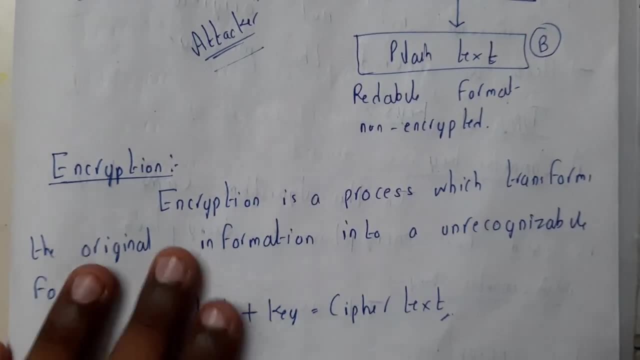 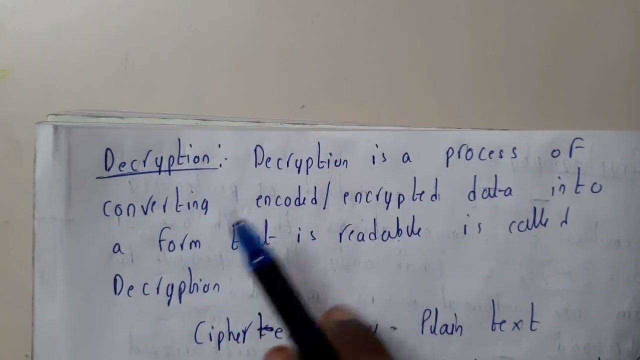 into an unrecognizable format. so here it is converted into unrecognizable format. so plain text plus key is equals to cipher text. fine, so when we add a key plus a original text, we will be getting a cipher text. so what is decryption? opposite of it, decryption is a process of 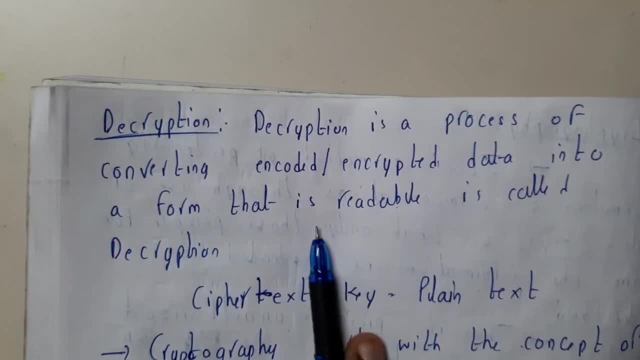 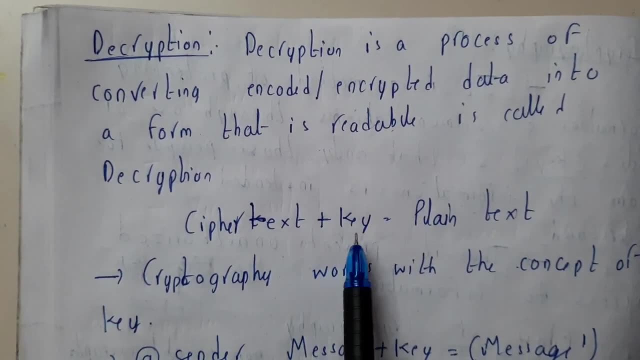 converting encoded or encrypted data into a form that originally it is readable is called as decryption. example: it will be cipher text plus key equal to plain text. so if the key is different it will be plus, if it is same, we will be subtracting the key. that's it. i hope everyone understood there. 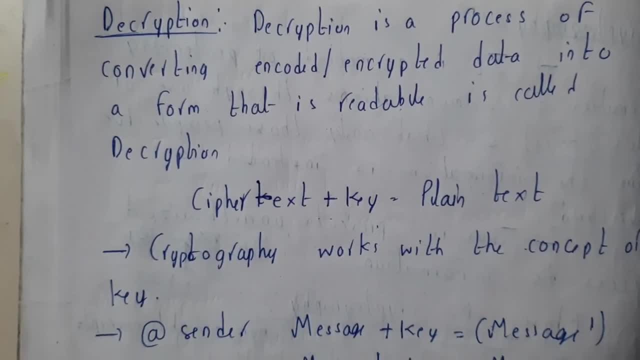 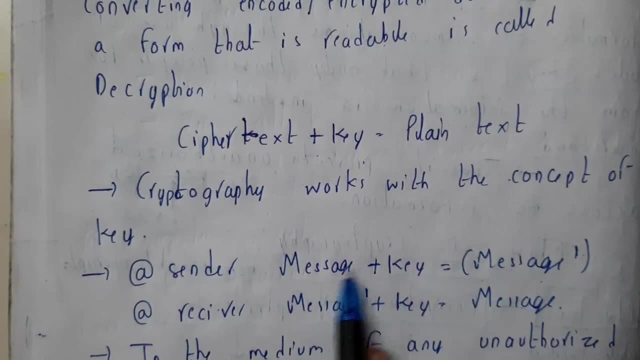 are two types of keys also we'll be discussing, don't worry. so basically, cryptography works with the concept of keys: sender message plus key equal to message dash, which is of some other message. if it is high, it will be by, like that. like it will not be by, it will be with some special characters. 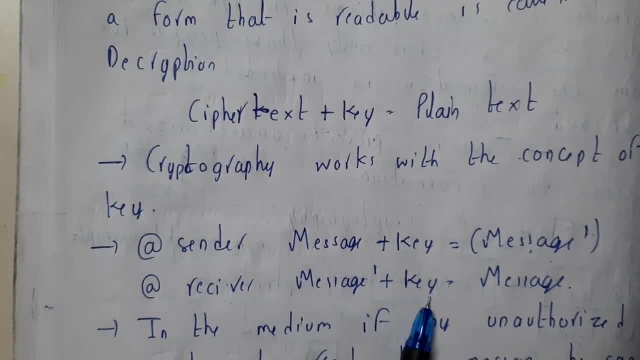 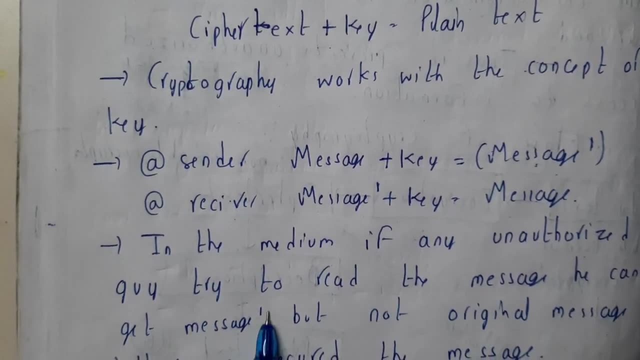 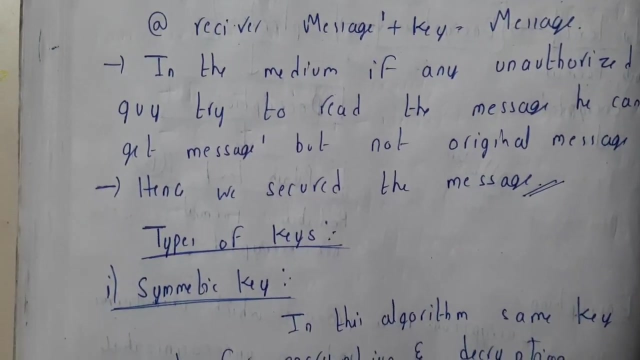 that's it. so. receiver: it will be message dash plus key. it will be getting the original message in the medium. if any unauthorized guy tries to read the message, he gets the message, message dash, but it is not the original message. hence we achieved the data security or message security, fine. so there are two types of keys, guys. one is symmetric key. 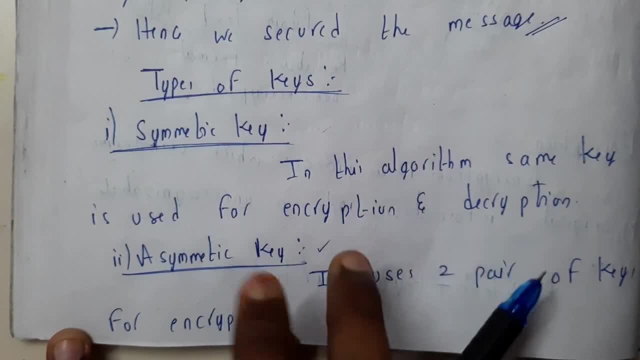 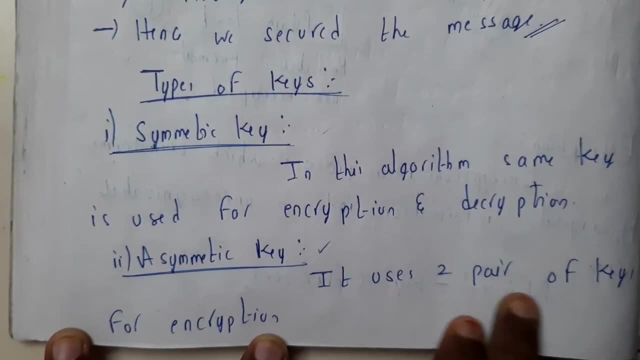 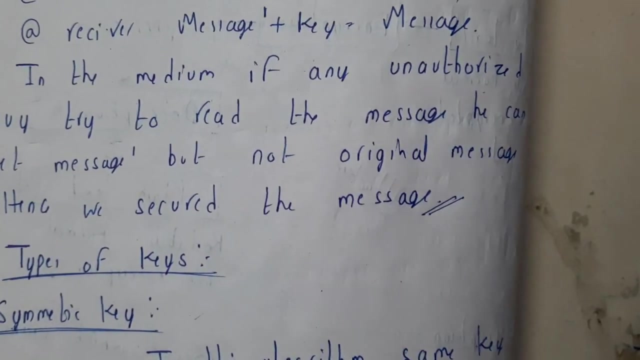 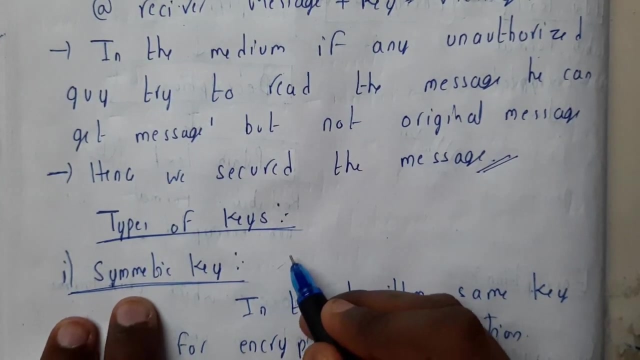 and asymmetric key symmetric. so symmetric means similar. so in this algorithm, same key is used for encryption and decryption, whereas asymmetric: it uses two pairs of different keys for encryption and decryption. fine, i hope everyone got a small. if you ask me what, what will be the example for it? okay, so for symmetric, symmetric it can be. 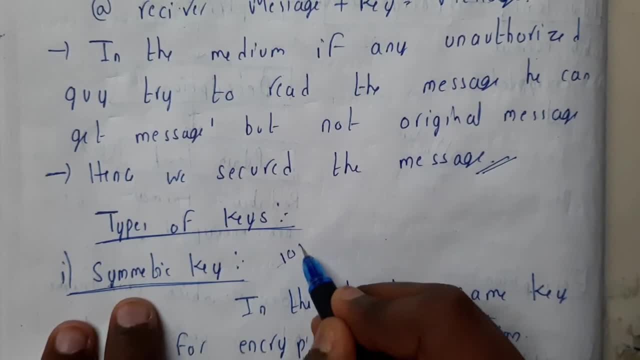 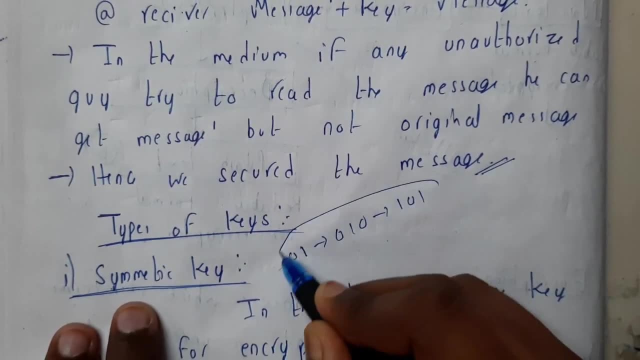 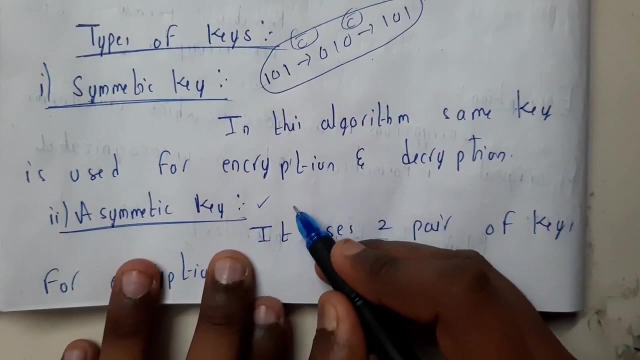 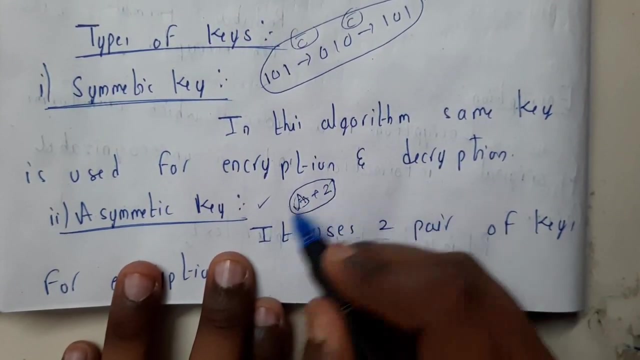 complement operation. so if i send 001 in the medium it will be 010 and at the end, just complementing it, we gonna get 101. so here i use the same key: complement, bar, complement, fine. whereas in asymmetric we can use a small trick. guys, this is popular in some, algorithms are there for this. so if you enter a litter,